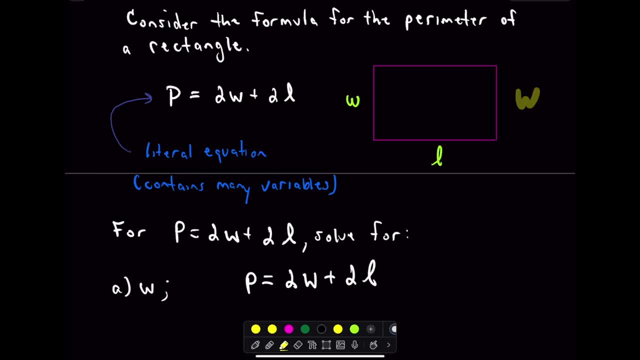 and this L, We have- quote-unquote- many variables. This is what's known as a literal equation And, at least in my experience, I don't remember too often running into situations where they were like, hey, this is a literal equation, So I don't think this terminology is going to be that. 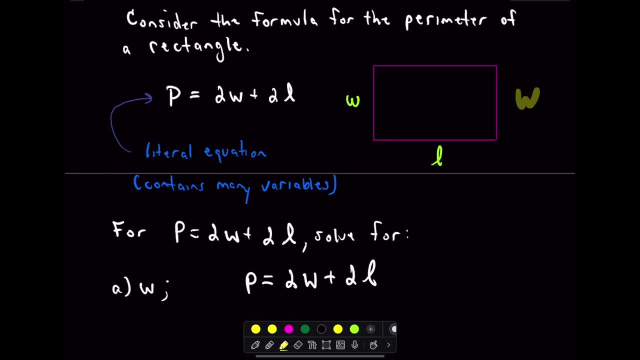 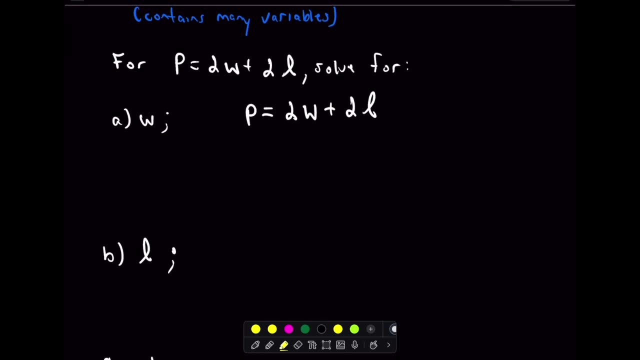 important. But hey, just be aware of it. But I don't think you'll encounter it that often. Okay, let's talk about solving for variables. So I'm going to take my perimeter formula and I'm going to solve for W in part A and I'm going to solve for L in part B, And you'll see. 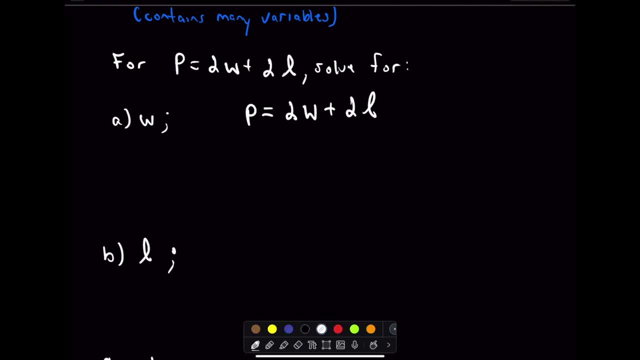 those are very similar, at least in this case. Now, when we want to solve for a variable, in this case W, I want to get that variable isolated. So eventually I want to come down to an equation that says W equals. and then I've got. 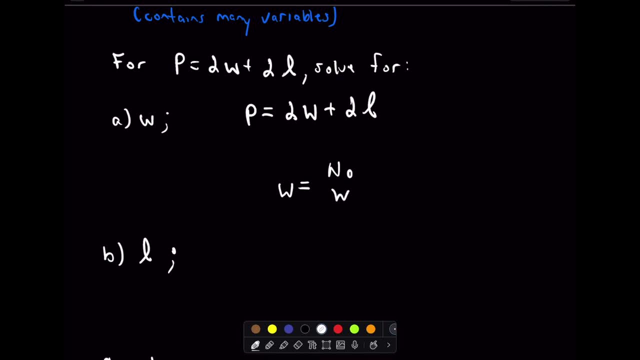 something on the other side of the equation. The thing that's important to me is: I want no Ws over there. As long as there's no Ws over there, I am perfect. So it just says we have to get the W isolated. So what I do is I look at my equation and I look at each term. So there's no W. 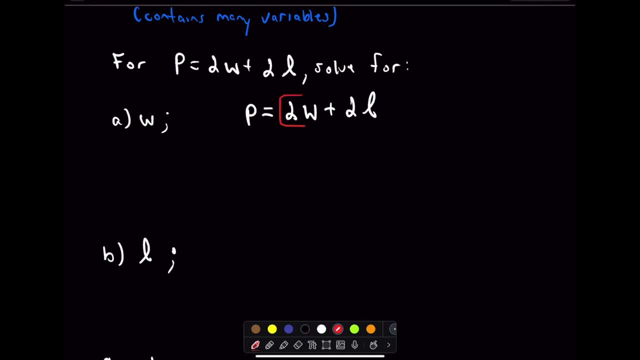 on the left, just that term involving P. I see this term 2W on the right, okay, But then I see this term 2L on the right that doesn't have a W, So I'm going to move that 2L over. Well, since I'm 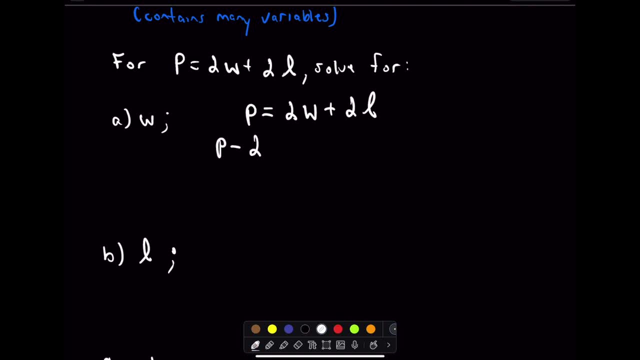 adding 2L to both sides. what I could do is subtract 2L from both sides And that's going to give me P minus 2L equals 2W, And now we can use the techniques that we've seen. So since I'm 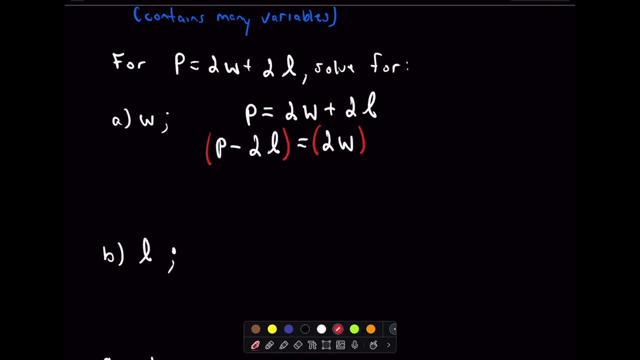 multiplying my W by 2,. I would simply divide both sides of my equation by 2, or, equivalently, multiply both sides by 1 half, And maybe I'll write 1 out here. but in general, I'm going to go through these a little. 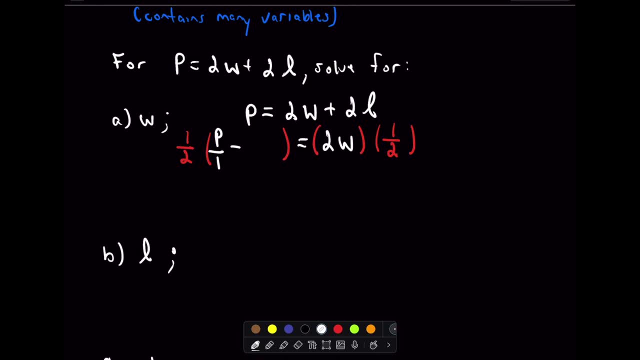 faster. So P, that's P over 1.. And then we had minus 2L, That's the same thing as 2L over 1.. Now when we distribute right, so 1 times P, that's going to give me P in the numerator. 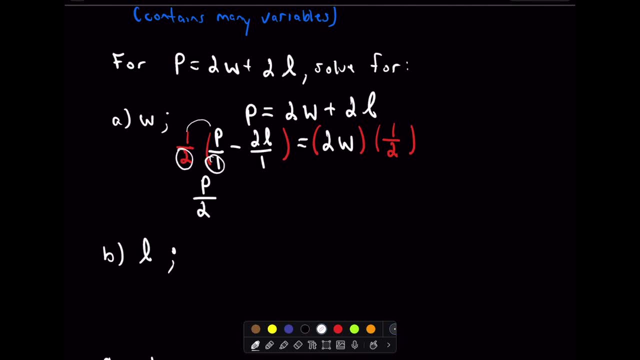 2 times 1 is going to give me 2 in the denominator And then I would have to distribute that 1 half to that. I would have to distribute that 1 half to that other, that other term in that parenthesis. So a positive times a negative is a negative. 1 times 2L is 2L And the denominator we have. 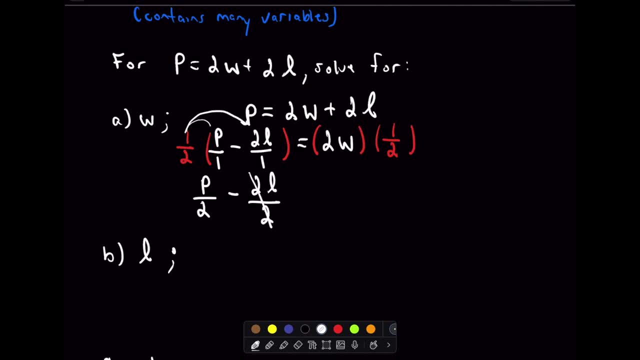 we would have 2 times 1, which is 2.. But notice, we could cancel those 2s out and really that's just going to leave us with minus L. Now on the right side, well, 2 times half, That's just going to be one w and we've got our solution. We have now solved for w And 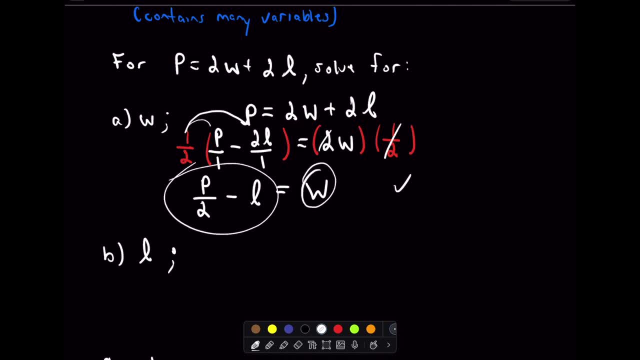 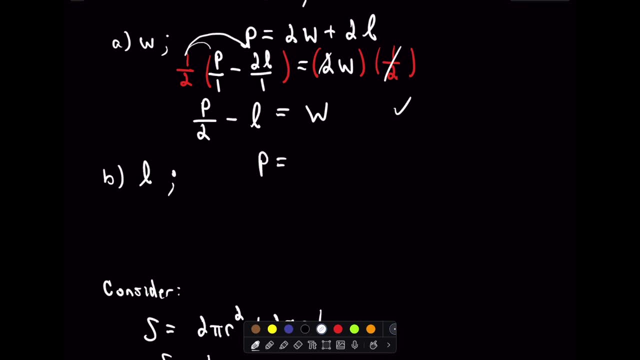 notice I've got w all by itself. There's other stuff on the other side but there's no w's, so I'm happy. Well, to solve for l. we would do the. you know, the same approach. Okay. so the only place I see an l is on the right. so I want to get rid of this 2w. that's. 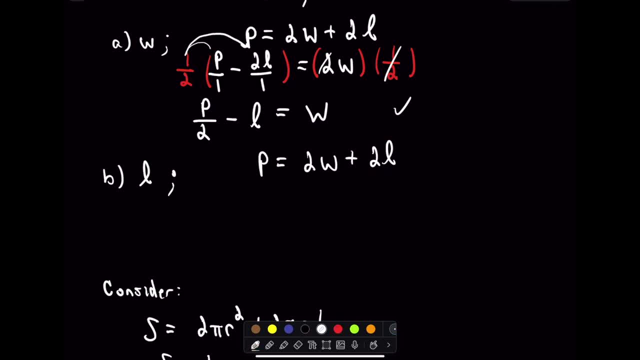 over there. So what I would do is simply subtract 2w from both sides- And again, let's make that a little better- And again, since we're multiplying by 2, I would simply divide both sides by 2 or, equivalently, multiply by 1 half And in much. 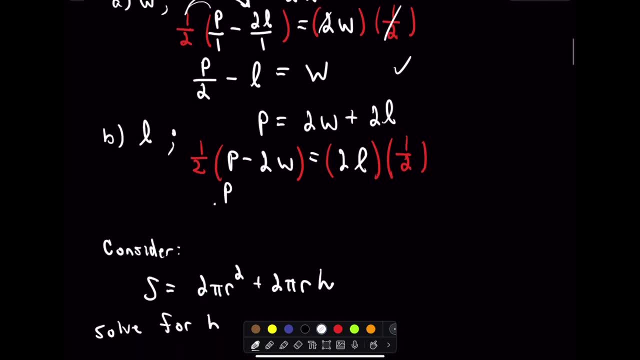 the same way when we distribute, we would be left with p over 2 minus w equals l, And we would be left with p over 2 minus w equals l. And we would be left with p over 2 minus w. And again, we've now solved for L. 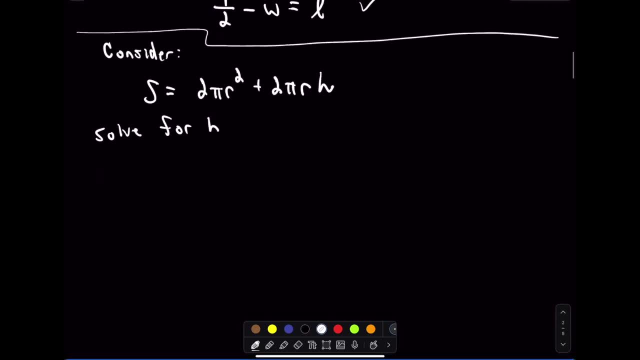 So let's look at another example here. So here I have that S equals 2 pi R squared plus 2 pi R times H. We want to solve for H. Again, same idea. There's no H on this term on the left, okay. 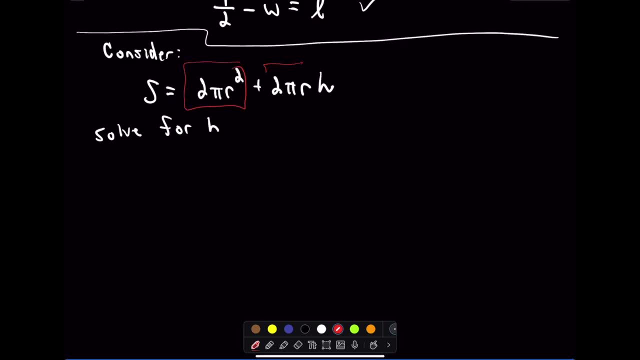 I see two terms on the right. The first one has no H. The second one does have an H, So I'm going to leave that term involving H. I'm going to leave that alone And I'm going to move this 2 pi R squared over to the left side. 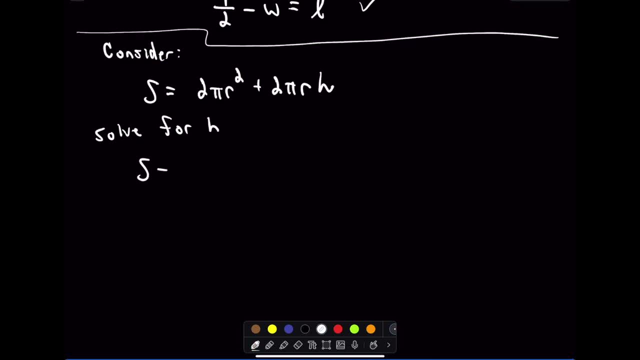 And I'm going to do that by subtracting. So I would have S minus 2 pi times R. squared equals 2 times pi times R times H. Okay, we want to get the H all by itself. So think about this: 2 pi R. 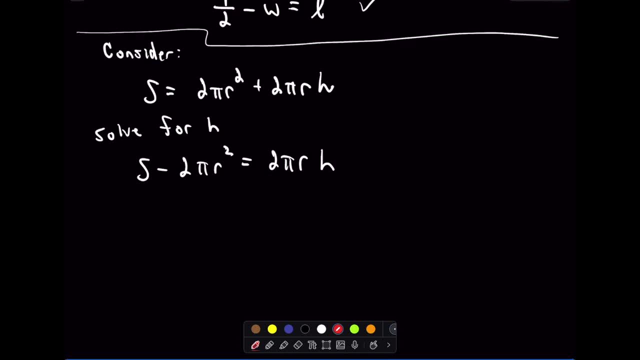 Think about that as being the constant that you're multiplying by. So what we're going to do is to get rid of it. I'm going to divide. I'm going to divide both sides by it. Well, dividing by 2 pi R is equivalent to multiplying by 1 over 2 times pi times R. 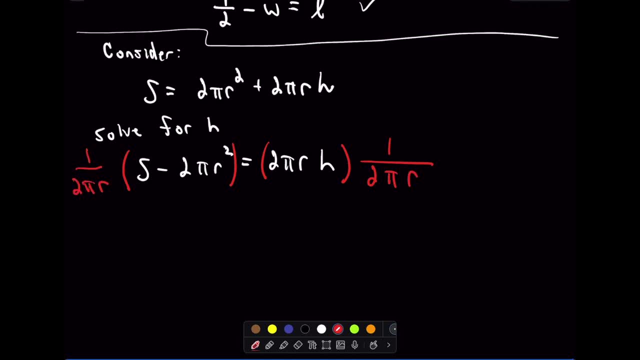 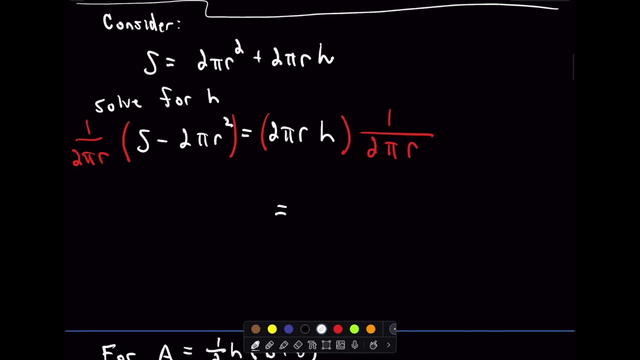 And then I would have to do that to the right side as well. Excuse me, the left side. I keep saying that We would have to do it to the left side as well. Okay, so if I distribute, I would get S over 2 times pi times R when I distribute. 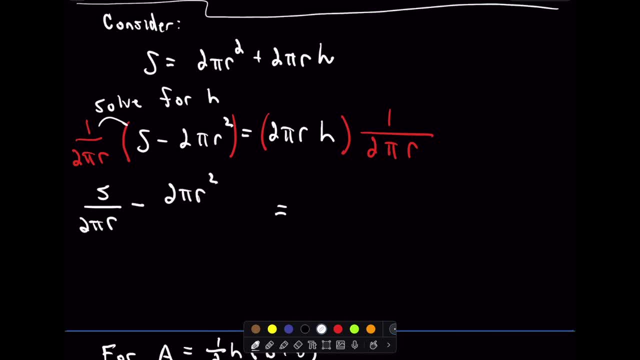 Minus: okay, I would have 2 times pi times R, squared all over 2 pi times R squared. Minus: okay, I would have 2 times pi times R, squared- all over 2 times pi times R. So I'm just distributing to that second term. 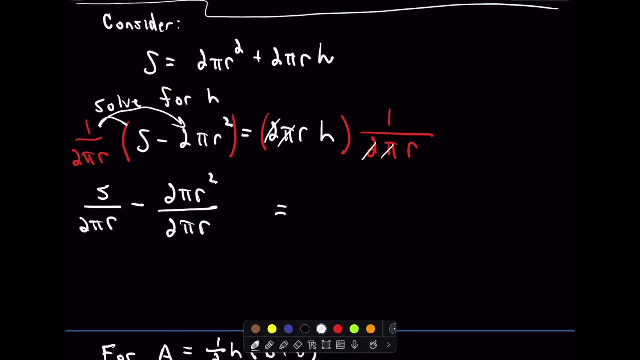 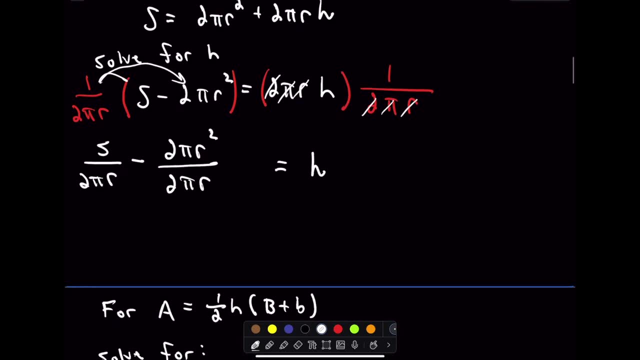 Now on the right, the 2's cancel, the pi's cancel, the R's cancel. That's the whole reason why we multiplied by that was just to get that H all by itself. Now on the left, there's really nothing to simplify in that first term. 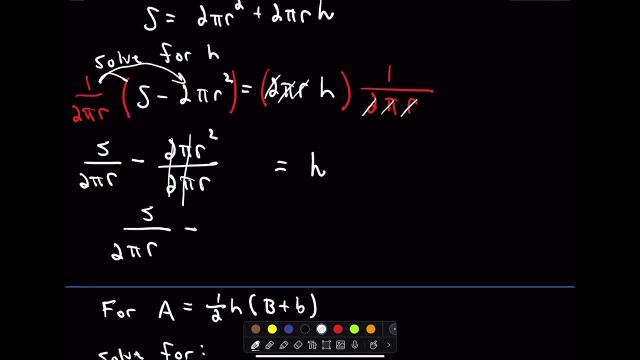 On the right: the 2's cancel, the pi's cancel. We would be left with R squared over R, but R squared over R, that's the same thing as just R. So my second term: I'm just going to be left with minus. R equals H. 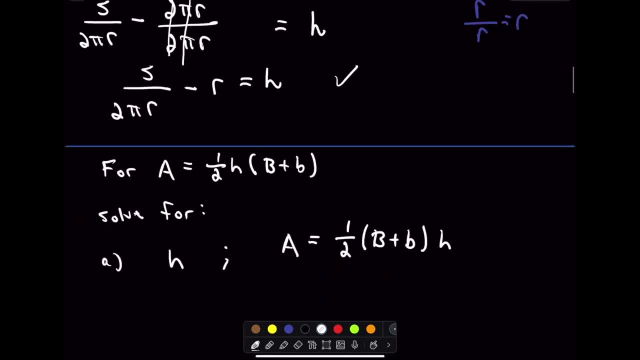 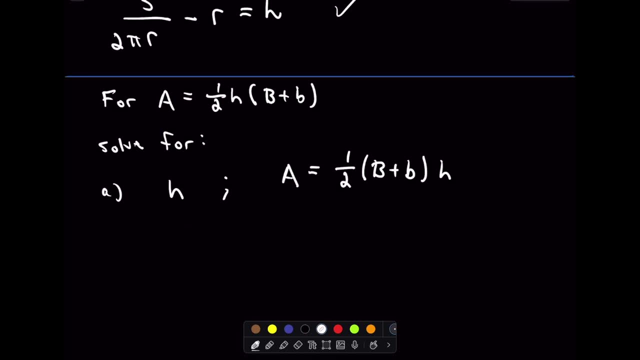 And again, we have now solved for H. Okay, so let's see here a couple more. So here we've got A, the area equals 1 half little h times this quantity capital B plus little b. And again a couple examples. 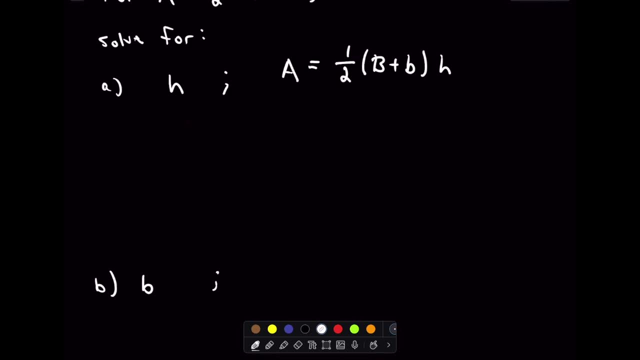 Part A, we'll solve for H. In part B, we will solve for little b. All right, so what are we going to do here? So I'm multiplying, I've got this 1 half, I've got this quantity b plus b, and then I see my H. 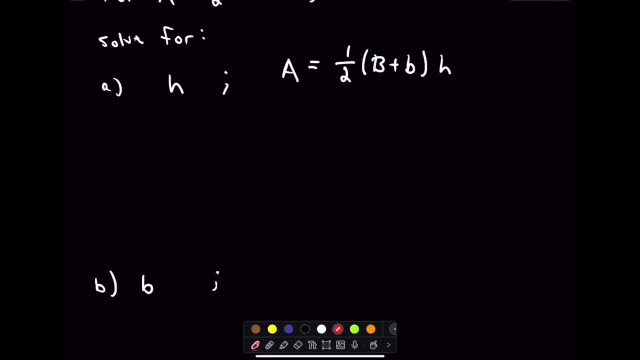 Now I want to get the H by itself, which means I need to get rid of that, the 1 half and the quantity b plus b. So the way that I would do that. let me give myself a little more space here. 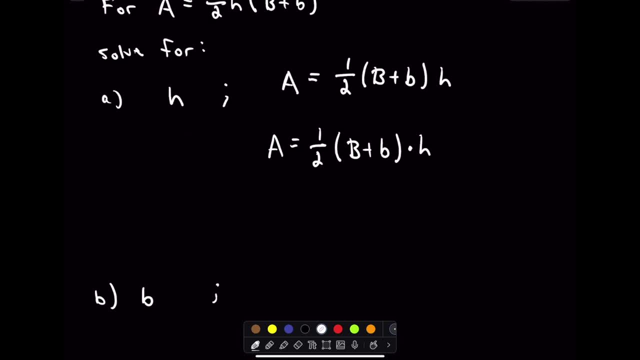 I'm either just multiplying or dividing by what I don't want to be there Is what I'm thinking. I don't want the 1 half to be there, So I would multiply both sides by 2.. And since I'm multiplying by this quantity b plus b, I'm going to divide by that quantity b plus b. 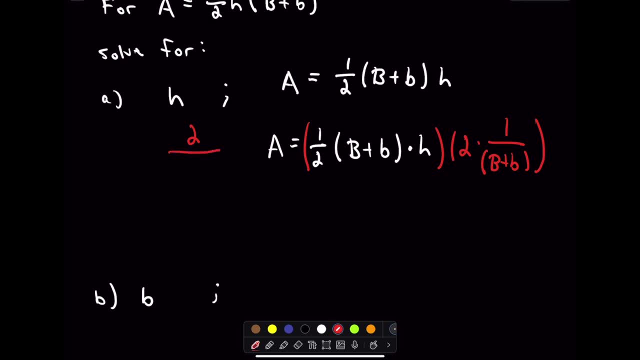 And that's what I'm going to. multiply both sides of my equation by And notice, if I take 2 times 1, that's just going to give me my 2.. So on the left side there's not a lot to do. 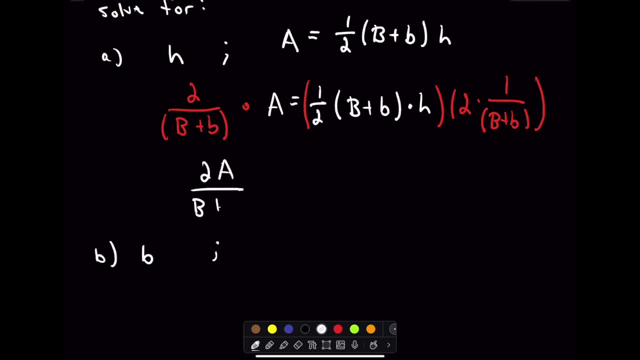 That's 2 times capital A over capital B plus little b. And notice on the right side again, the 1 half and the 2 are gone. That's what we wanted. This quantity b plus b is going to get canceled with this quantity b plus b. 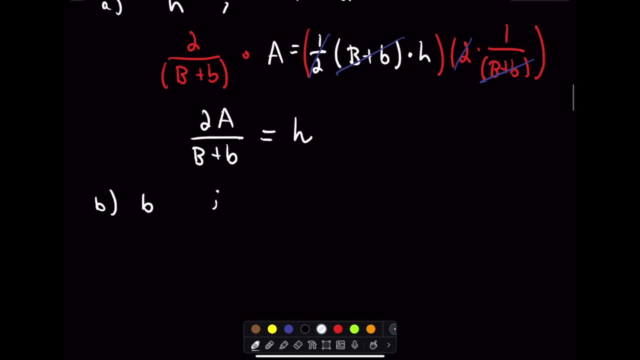 And then we're just simply left with H, and that's what we wanted. Okay, so let's look at one more of these. Okay, so, in the next one we want to solve for little b, So I want to get this little b all by itself. 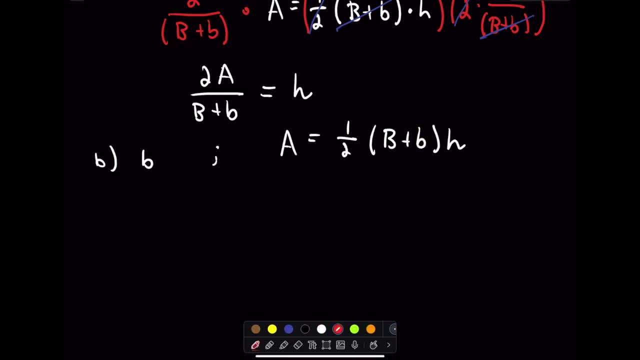 Well, what can we start getting rid of on the right side? Well, let's see A couple things I could get rid of. To get rid of that 1 half, I could multiply by 2.. And to get rid of the H, I could multiply by 1 over H. 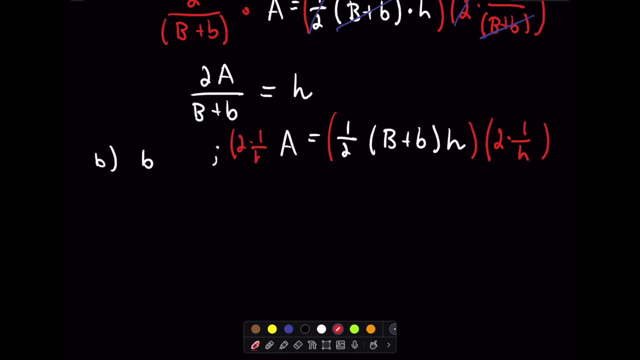 So I would have to do that to the left side as well. Now on the right side. I would have to do that to the left side as well. On the left again, this is 2 over 1 times 1 over H times A over 1.. 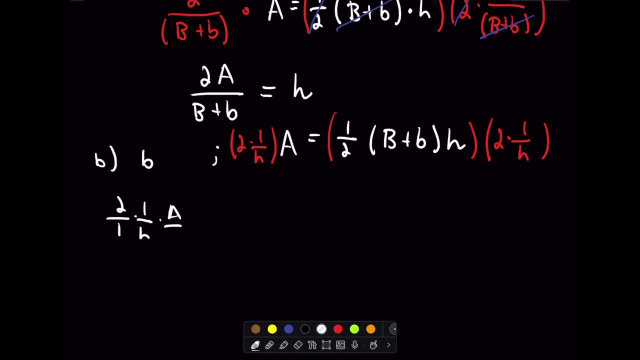 That's what all of this really says. So you're going to get 2 times A in the numerator and just H in the denominator, So that's going to be 2 times A over H. Now on the right side, the 1 half and the 2 cancel the H and the 1 over H cancel. 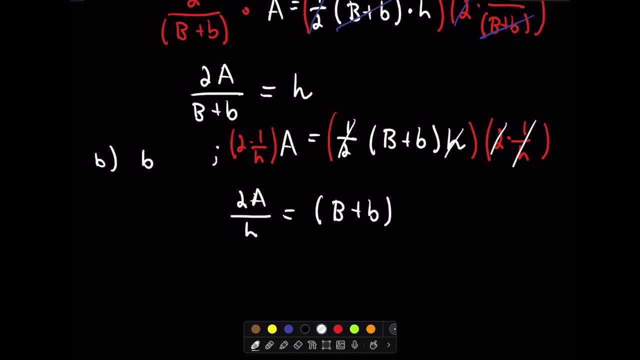 That's just going to leave me with b plus b. Notice I've put it in parentheses, But really there's just a 1 here And if I distribute that 1, I'm just going to be left with what is inside the parentheses. 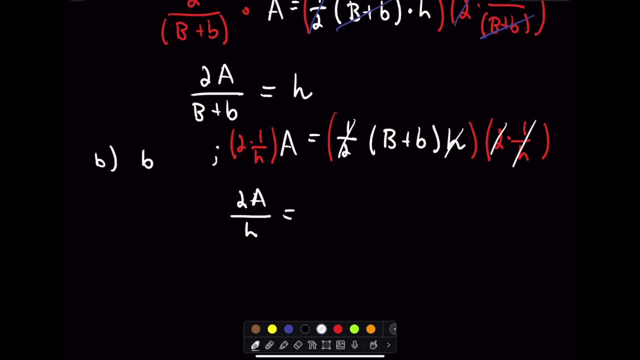 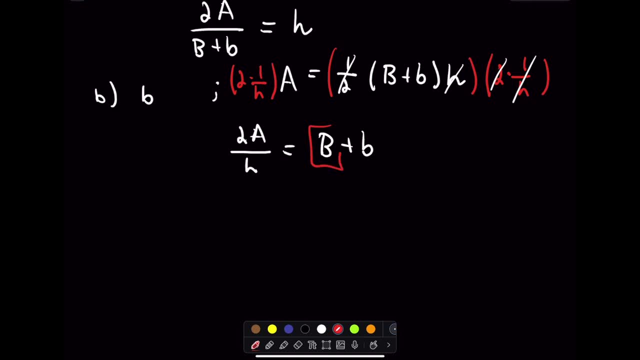 So I'm just going to be left with capital B plus little b, And if I want to solve for little b, well, I want to get rid of capital B. So I'm going to subtract that from both sides. All right, And we have now got it. 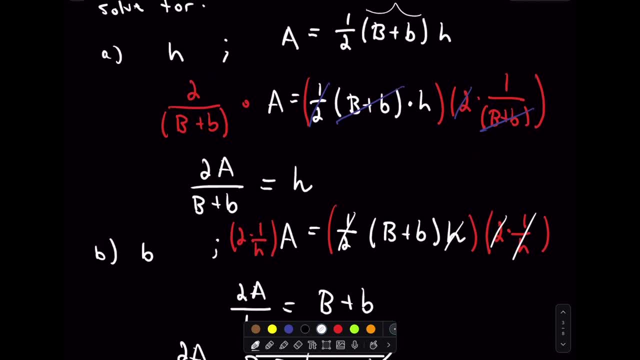 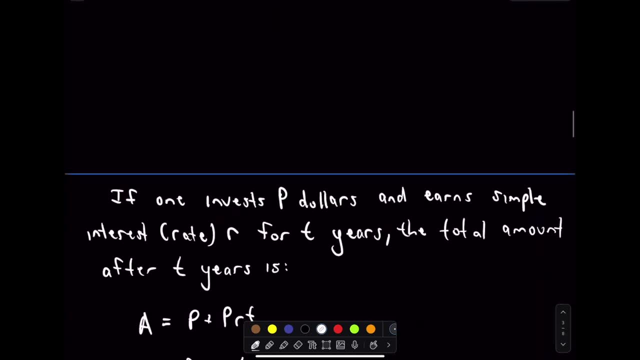 So again, the thing that's a little bit different in that example is: hey, we've got this stuff in parentheses that we have to maybe take an extra step or two to deal with. OK, Let's try to set up some examples. 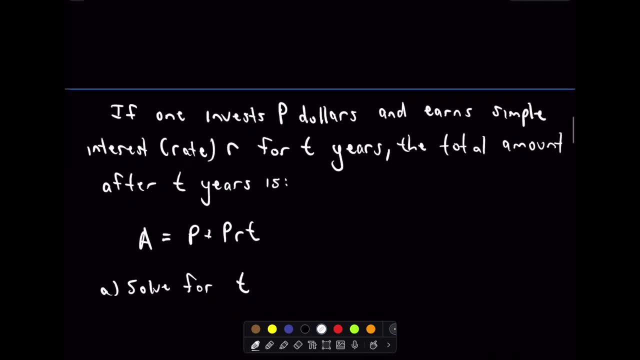 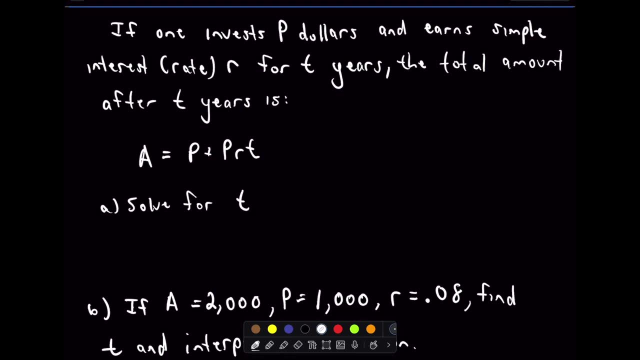 And maybe I can work all the way through them Or maybe we'll at least get them going OK. So this is a very applicable situation. Money right- This is something that finances. This is done day in, day out. So if one invests P dollars, that's your principle. 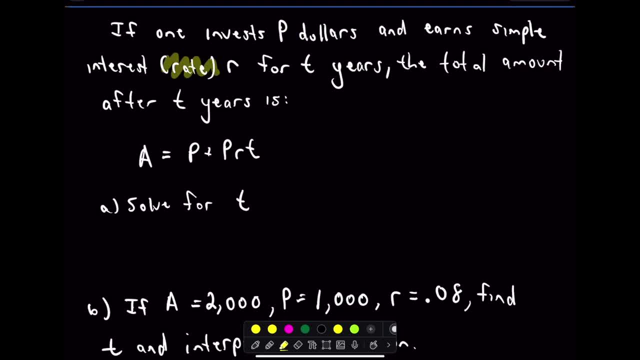 That's what you start with And earns Simple interests at a rate are for T years. So maybe you earn 10% per year, 20% per year, The total amount after T years it says the total amount is going to be. 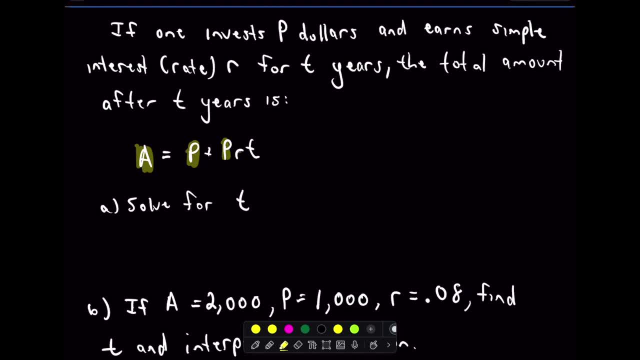 it's the principle you started with, plus we'll take the principle times the rate, times the time. This second part just amounts. the represents the amount of interest you've earned. So we'll take the amount of interest we've earned plus our original amount that we started with. 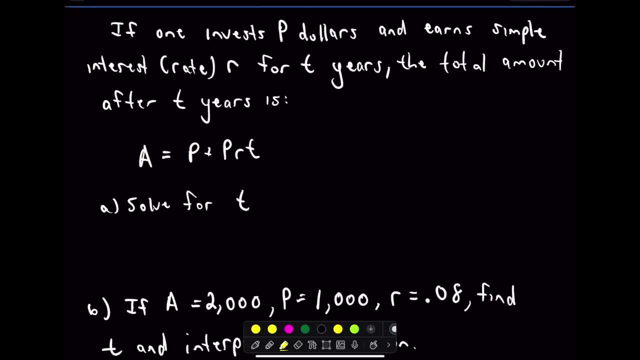 That's going to give us our total amount. OK, Part A: we want to solve for T. Well, let's do that. If we solve for T, the only place I see a T is in this second term on the right side. 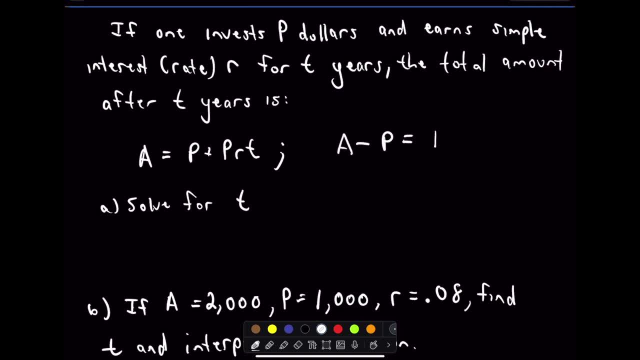 So I could subtract capital P from both sides. And now, if I want to solve for T again, I think: well, I'm multiplying by P times R, I'm going to divide by P times R. Well, if I do it on the left, I have to do it on the right. 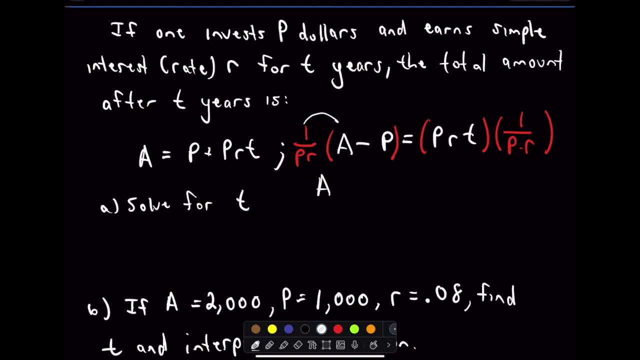 And if I distribute I would have A over P times R minus capital P over P times R. But notice, those P's would cancel And that's just going to leave me with 1 over R. Now, on the right side, the P and the P cancel, the R and the R cancel and we're simply left with T. 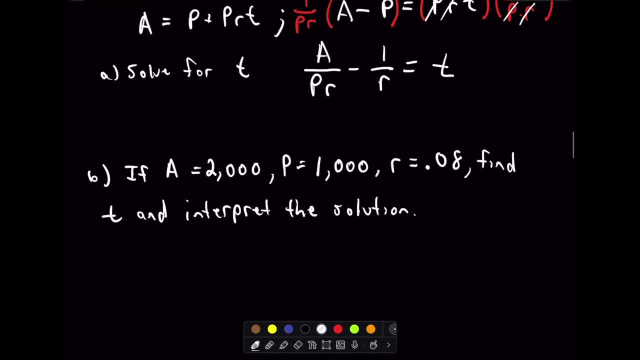 So we've now solved for T. So part B says: OK. so if the total amount of money that we end up with is $2,000, if the principal we start with is $1,000 and you're earning an interest rate of 0.08 or 8% per year, we want to find T and interpret that. 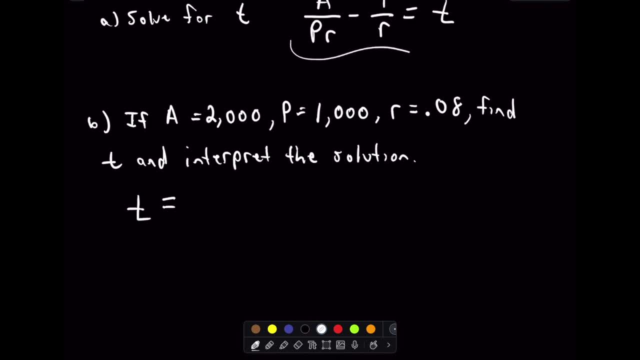 OK, so we want to find T. So I'm just taking this equation that I just found, And again I'm going to put the T first, And it says we have A That's going to be $2,000.. So I'm just reordering this. 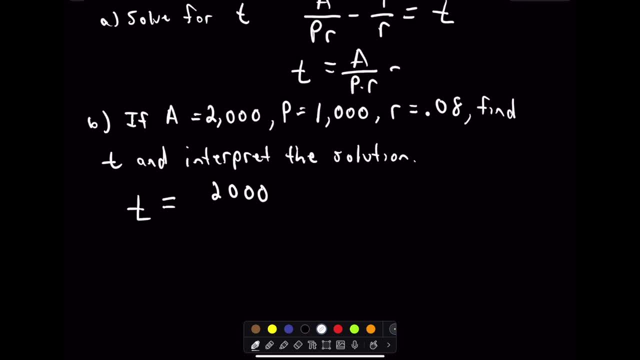 T equals A over P times R Minus 1 over R. I'm just reordering this And now I'm filling in those values. So it says P, that's going to be equal to 1,000.. That's being multiplied by R, which is 0.08 minus 1 over 0,, excuse me, 0.08.. 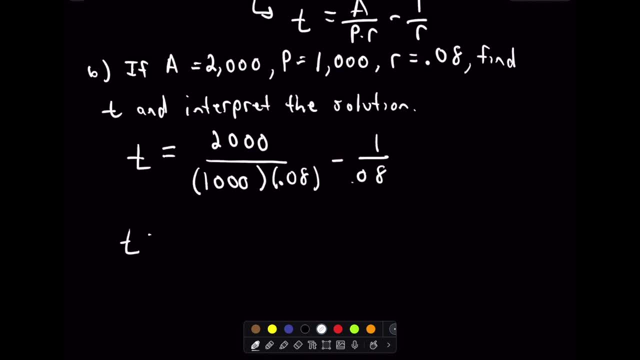 It says that's going to be our value for T. And notice we could simplify: 2,000.. Over 1,000.. That's just 2. Divided by 0.08 minus 1 over 0.08.. 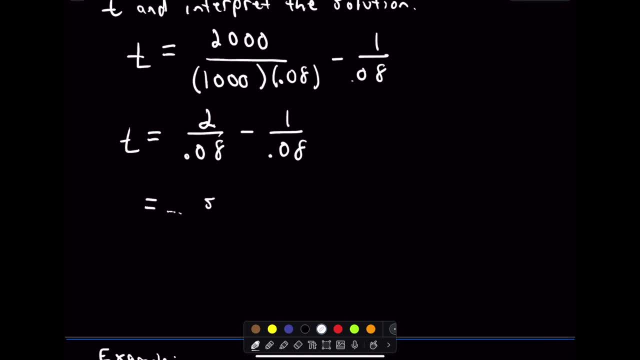 And I'm going to let you simplify this. So just put it into a calculator is what I would do. I don't know. Let's go ahead and do it, Why not? I always say this. So let's see 2 divided by 0.08.. 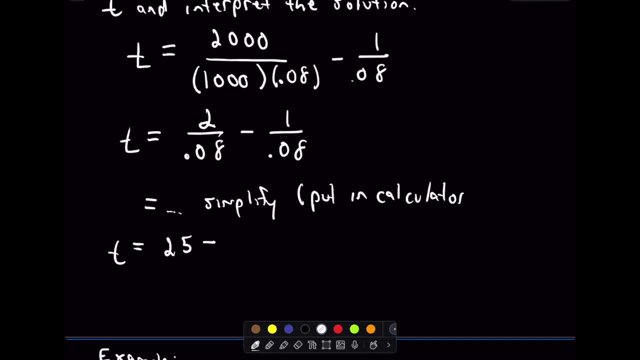 That's going to be 25 minus. let's see so: 1 divided by 0.08.. That's just 12.5.. 25 minus 12.5.. That's going to be 12.5.. So it says T equals 12.5.. 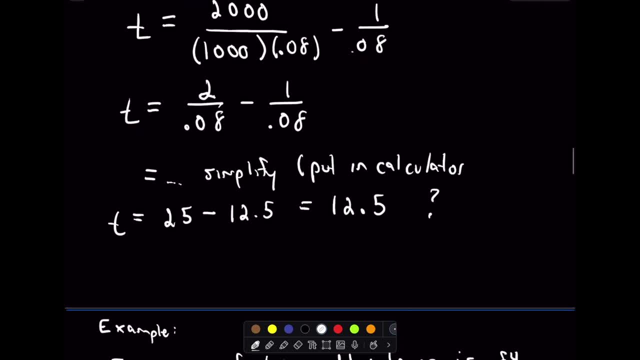 12.5 what? This is the interpretation. So it says it's going to take 12.5 years to earn $2,000.. Because that's how much we wanted to finish with: It's going to take 12.5 years to earn $2,000. 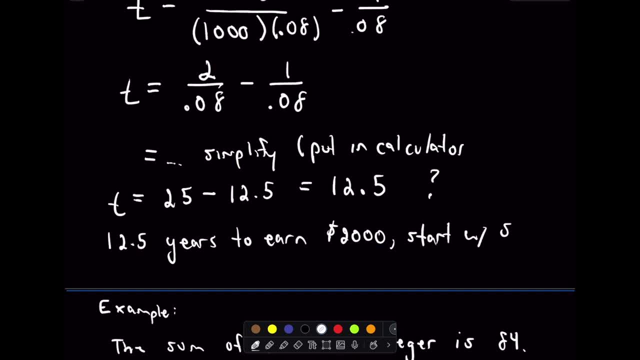 If we start with $1,000 and we earn 8% interest, I should say simple interest per year. Okay, That's what this number means. So we've solved for T. It has something to do with time. Well, it tells us how long. 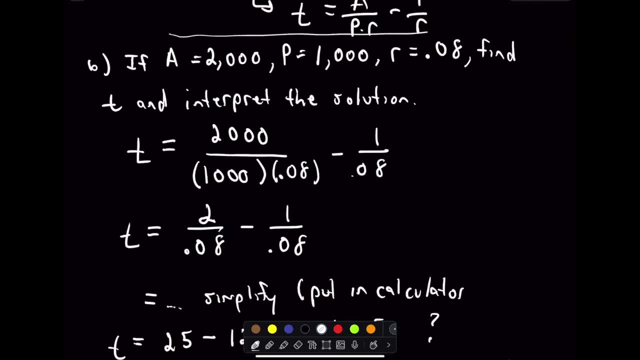 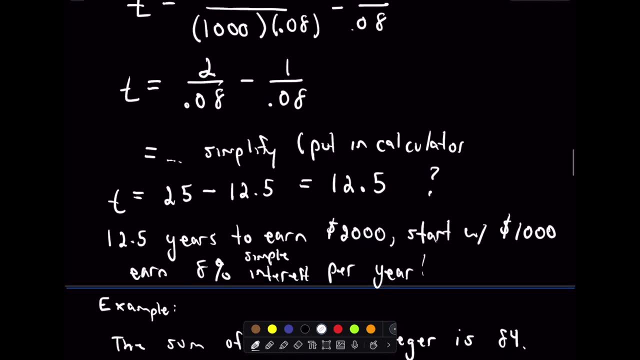 It's going to take to satisfy all of these other restrictions. We want the final amount to be $2,000.. We start with $1,000 and we're getting 8% per year. That's what it tells us. Let's just set up a couple more examples here. 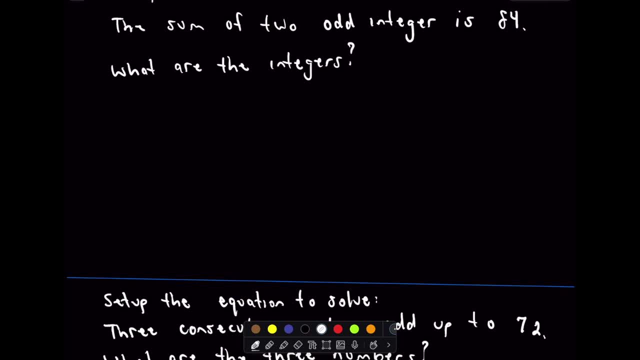 I'll let you finish these off. It says the sum of two odd integers is 84.. What are the integers? Now, of course, you could just start guessing and checking and probably coming up with these, But the point is, try to take these English phrases. 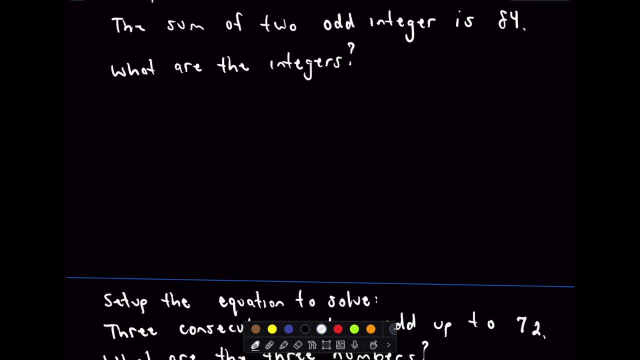 and write these in some sort of mathematical term, because eventually you're going to get to some situation that's too complicated just to guess and check. So let's think about our consecutive odd integers. So I want to write things generically because I don't know what these odd integers are. 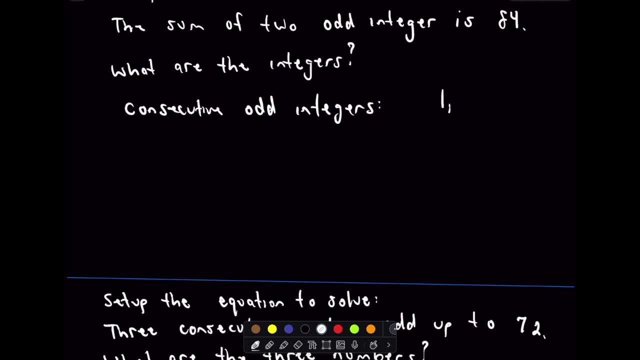 So let me think about numbers. in a row, I could write 1,, 2,, 3, 4.. Those are consecutive numbers, They're not odd. So let me try to think about this a little more generically, right? 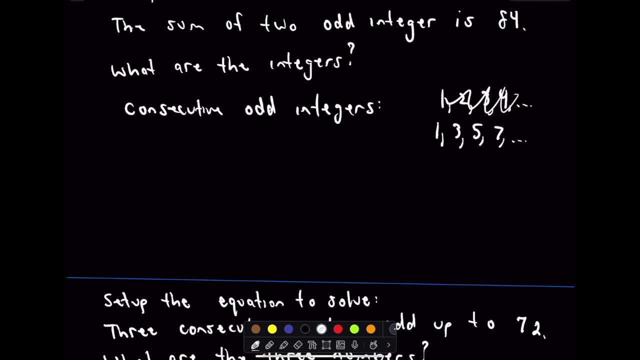 Those are consecutive odd integers: 1,, 3,, 5,, 7.. How can I write this generically? So the idea is, if I start with some number x, you know the next number, well, would be x plus 1, you add to it. 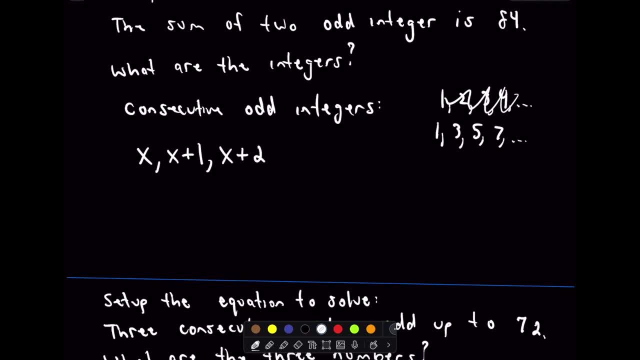 And then, to get to the next number, we would have x plus 2, et cetera, et cetera, et cetera. Now, let's assume that this number, let's assume that this one, this number's odd, 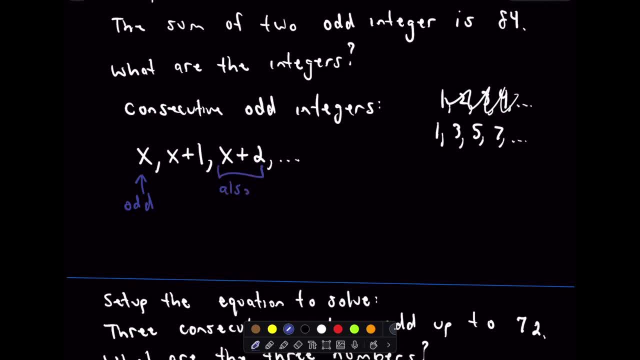 If that one's odd, that means this one's odd. Let's assume that this one's odd. Let's assume that this number is also odd And those are going to be consecutive, right? Those are odd numbers that fall one after the other. 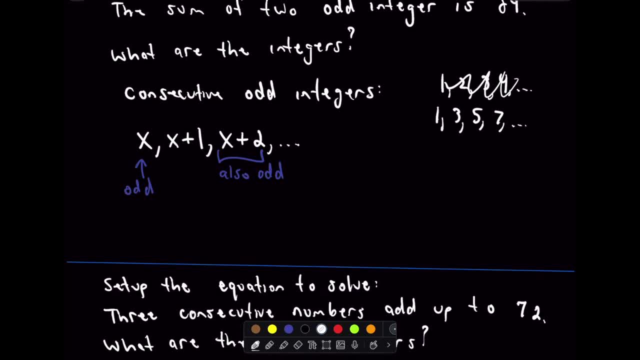 So now we're going to come up with our equation. It says the sum of two odd integers. So one odd integer is x. If we add that other odd integer, which is x plus 2,, it says that has to equal 84.. 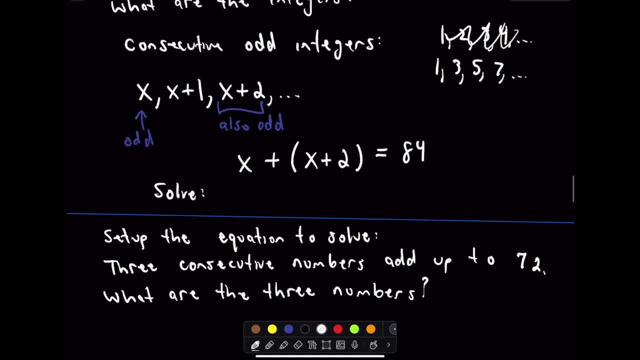 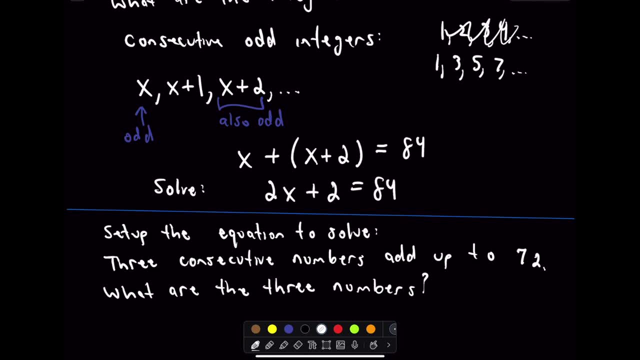 And now we would simply just solve this equation. Notice, we have x plus x, Which is going to be 2x plus 2 equals 84. And I'll leave this for you to solve And once you know that it's going to tell you one of the odd integers. 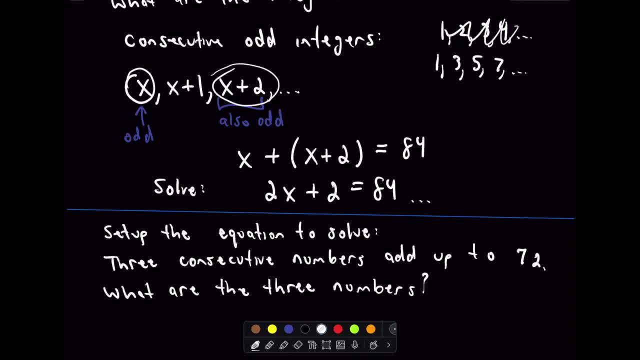 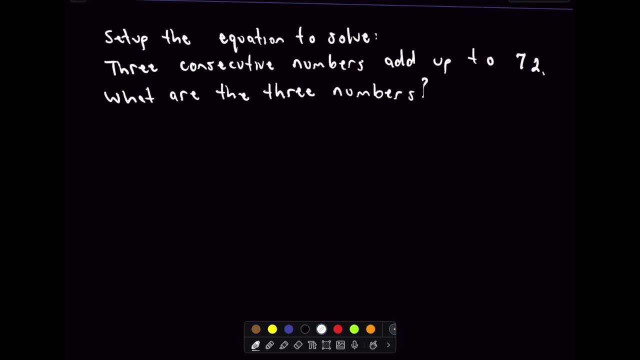 And then you could add 2 to that one to get the other odd integer. So that would be our solution. So in this question we've got three consecutive numbers that add up to 72. And we want to know what are the three numbers. 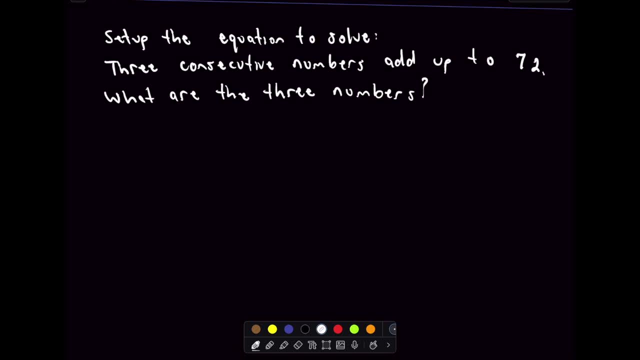 So this is very similar to the last question. Two differences. Now we have three numbers And notice they're consecutive, right? They're not even or odd, like the last one. The last one had to do with odd. Well, if my first number is x, my next number would be x plus 1.. 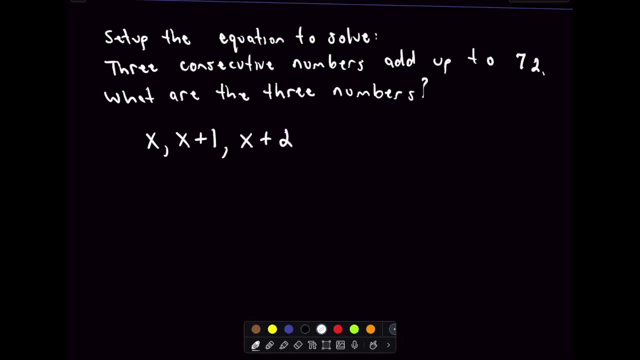 Well, my next number would be x plus 2.. Those would be three consecutive numbers. Well, to come up with my equation, it says: if we add those three numbers together. So I'll take x plus x plus 1 plus x plus 2.. 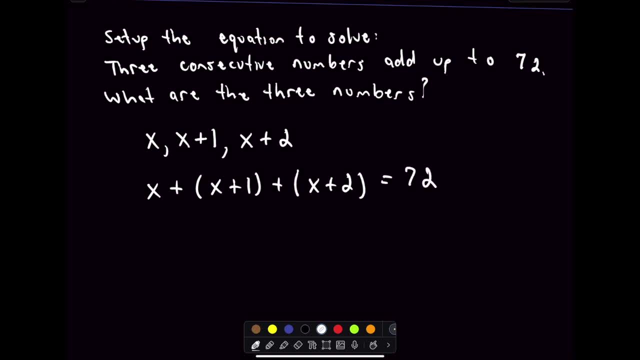 And we know, if we add those all together we get 72.. Now again, I know this question. you could just really guess and check and come up with these numbers. But the point is learning these techniques to go from phrases to mathematics. 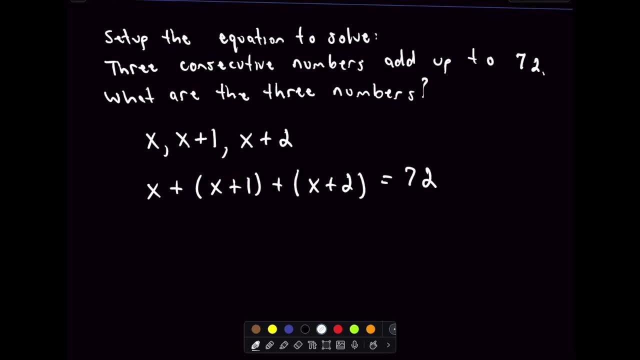 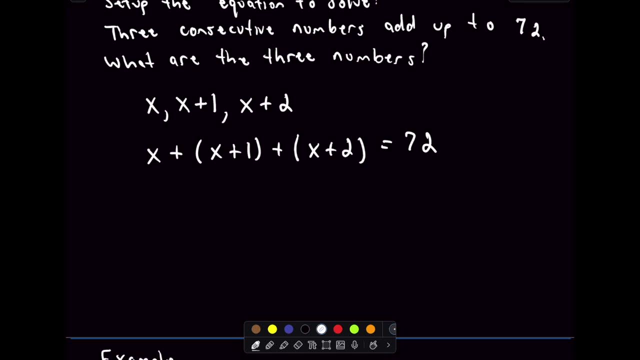 Because eventually you will certainly encounter situations where you can't just guess and check. You have to produce the equations, grind through them, come up with a solution. Okay, So on the left we could get rid of parentheses. combine like terms. 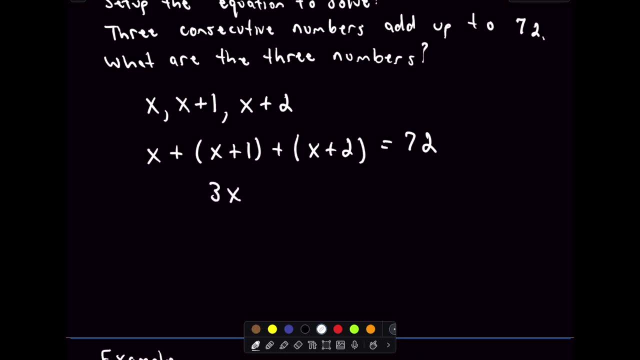 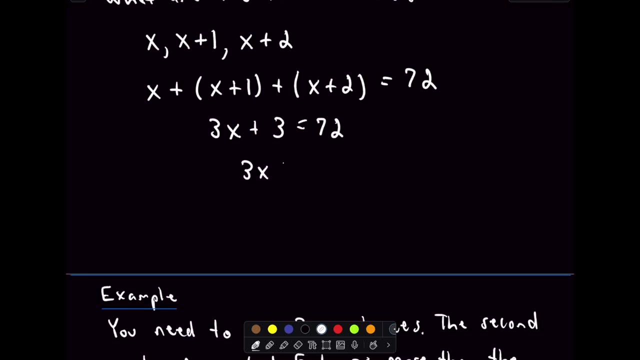 We would have x plus x plus x, which is 3x. 1 plus 2 is 3.. That equals 72.. We can subtract 3 from both sides. We'll get 3x 72 minus 3 is 69.. 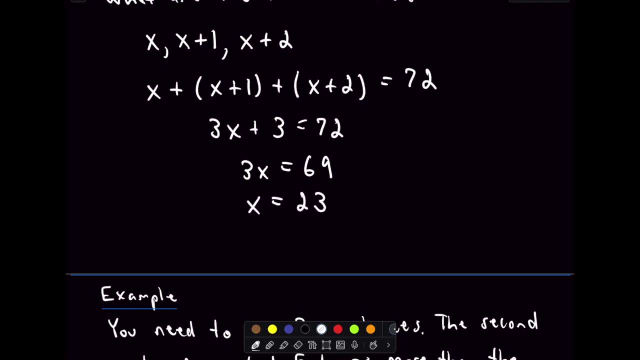 If we divide 69, divided by 3,, that's going to be 23.. So now it says that the numbers right. we always have to be careful Because if we just stop here and we say, well, x equals 23,, that doesn't tell me the three numbers. 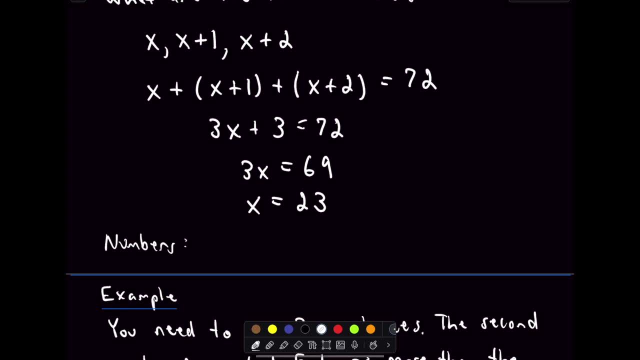 You're almost there. It says the smallest number is 23.. The next number must be 24.. And then the last number must be 25.. And you can add those up and verify. hey, we do get that. those add up to 72.. 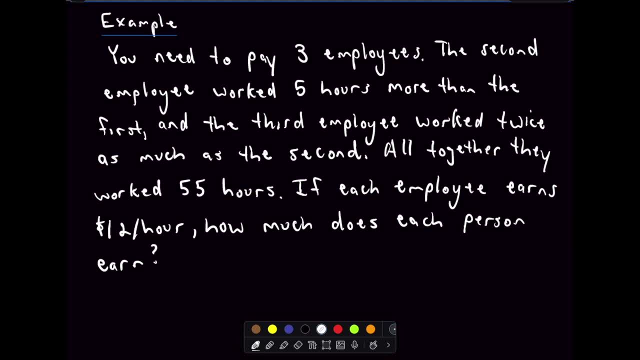 Okay, Last example: So you've got to pay three employees. So it says the second employee worked five hours more than the first. We don't know how many hours the first person worked And the third employee worked twice as many as the second. 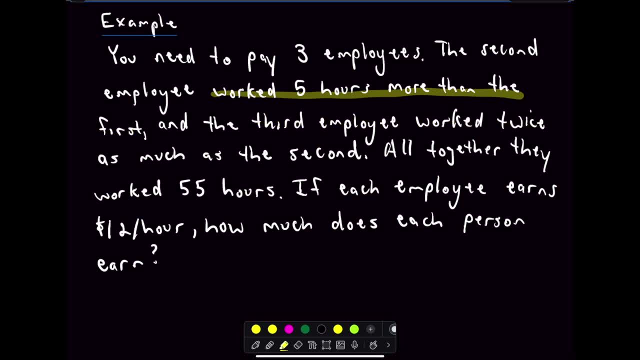 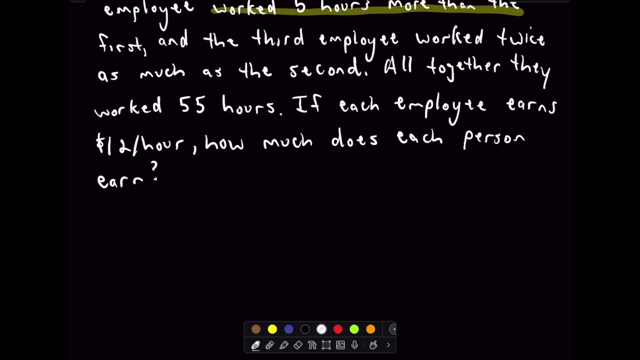 Okay, So all together they worked 55 hours, And we want to know if each employee earns $12 an hour, how much does each person earn? So to me, really, the question is: how many hours? you know? how many hours did each work? 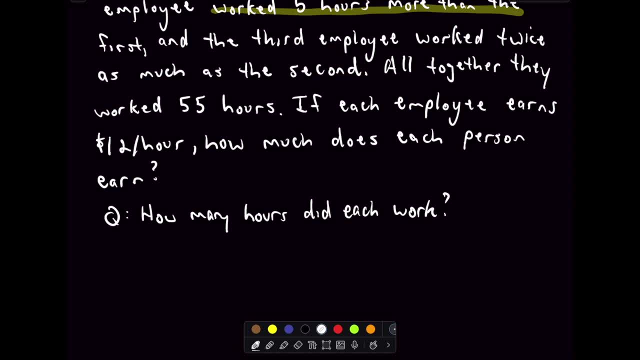 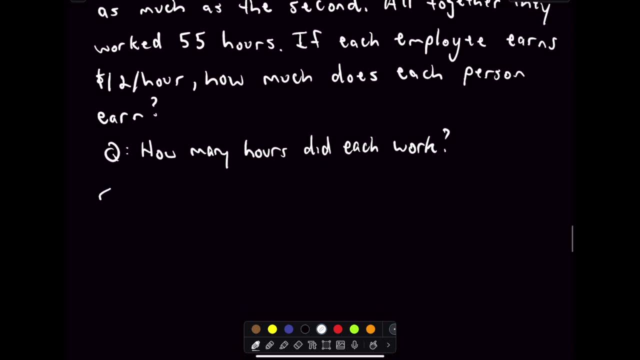 At least I should say to me. that's kind of the hard part, Because once I know how many hours each person worked, I can just multiply that by 12.. So let's see, there's employee one, there's employee two, there's employee three, and this is going to represent the number of hours worked. 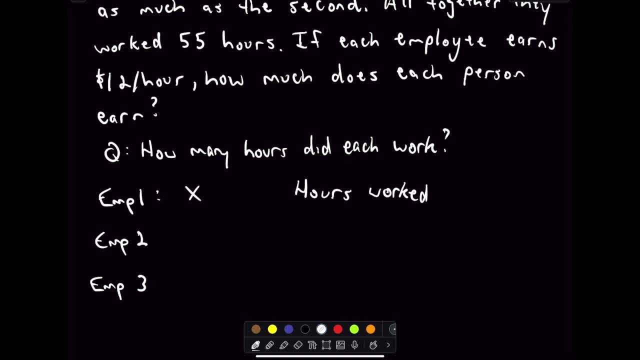 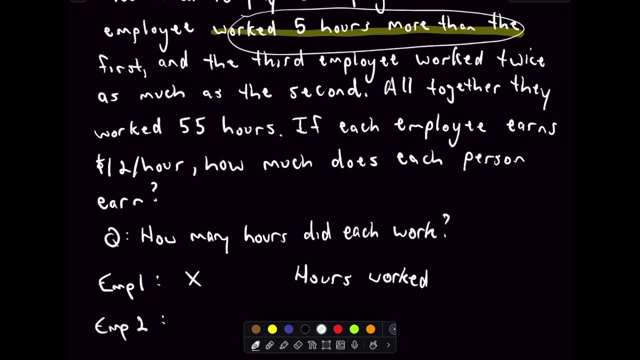 Okay, I don't know how many hours the first person worked, So I'm just going to label it something generic. I'm going to label it as X. Well, I know that the second employee worked five more hours than the first. Well, I would just add five to the number of hours of employee one to get the number of hours. 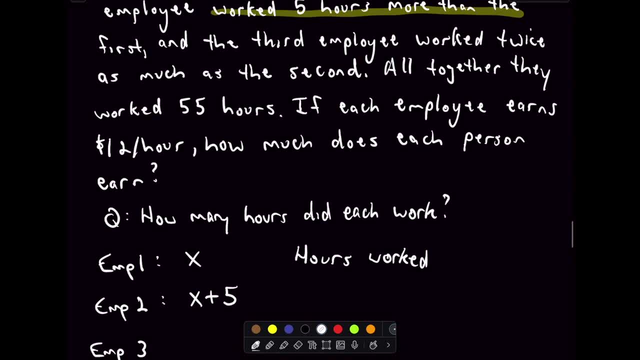 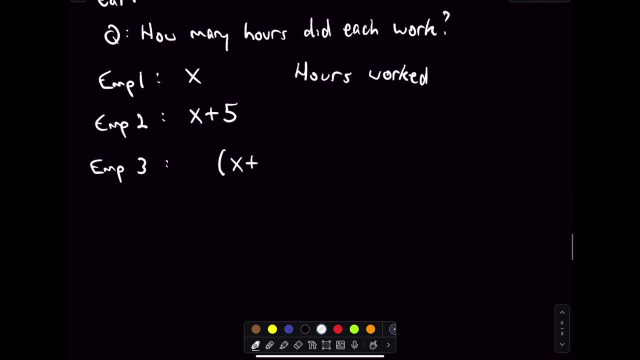 And then it says the third employee worked twice as much as the second. Well, we would have to take the number of hours that the second employee worked and we would have to double that. Be careful, Make sure that you do put that X plus five in parentheses, because if you don't distribute the two, you'll have a problem. 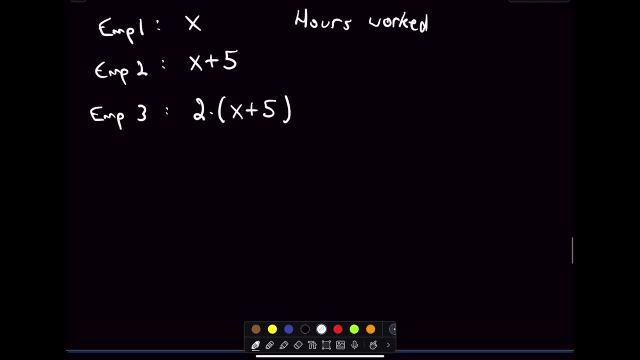 Well, we know that the total hours worked is 55. So I could simply take X Plus X plus five plus two times X plus five, And we know that has to equal 55. So again, I've kind of gone from the English now to the mathematical equation that I have to solve. 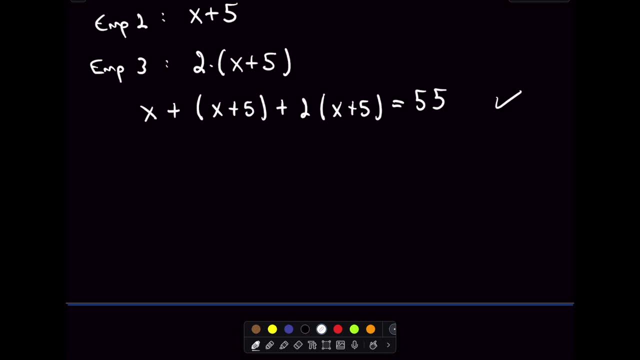 So now I'm- you know I'm- in the world of mathematics. How do we solve this? Well, I'm going to get rid of the parentheses. So I've got X plus X plus five. Now notice on this third term on the left. we have to distribute the two. 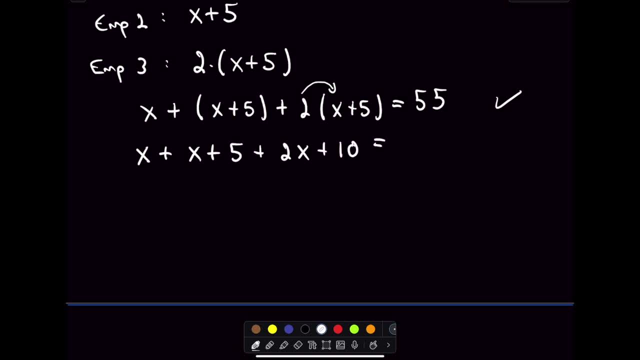 So we'll have two X. Two times five is 10.. On the left side, if we combine our like terms- X plus X plus two X, that's going to be four X, And then the five and the 10,, that's going to be 15.. 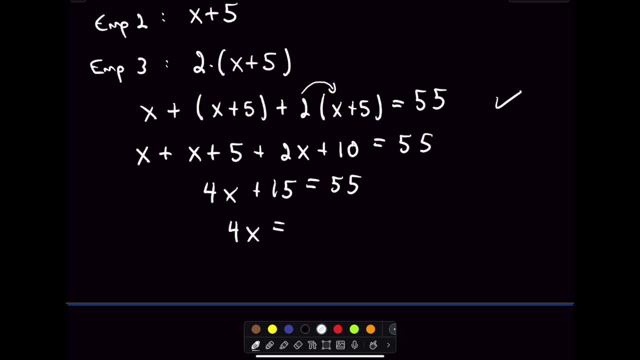 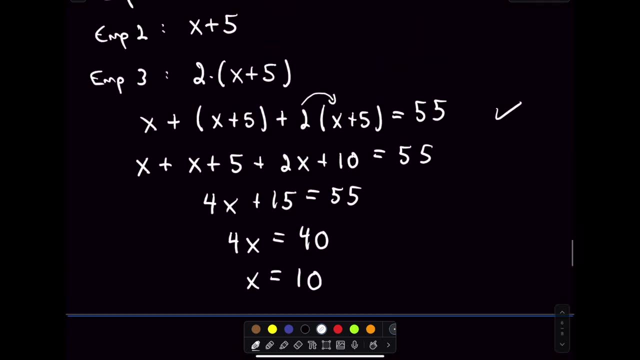 Well, I can subtract 15 from both sides. Fifty five minus 15 is 40. And then 40 divided by four, that's going to be X equals 10.. So now that Tells me that the number of hours worked 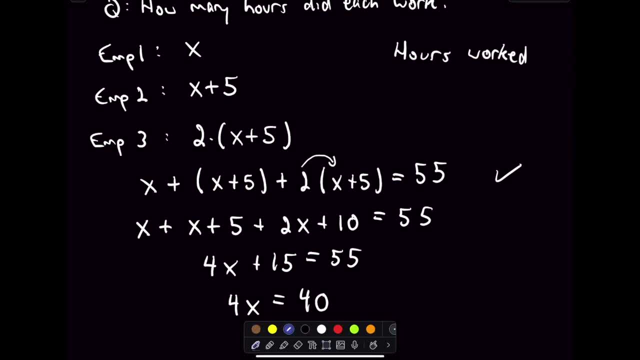 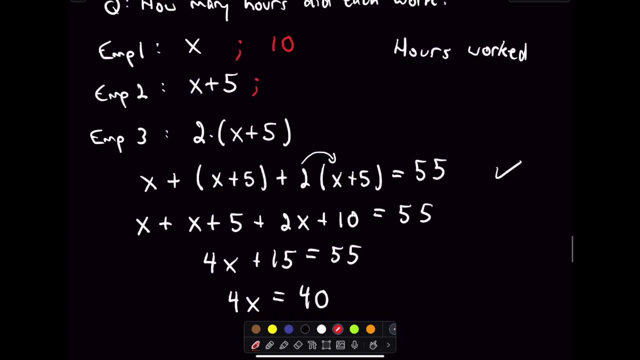 So that tells me that the number of hours worked OK. we said that the first person worked 10 hours, because that's what X equals. Well, that means that the next person worked 15 hours because they worked five more, And the last person- while we double it, that person- worked 30 hours. 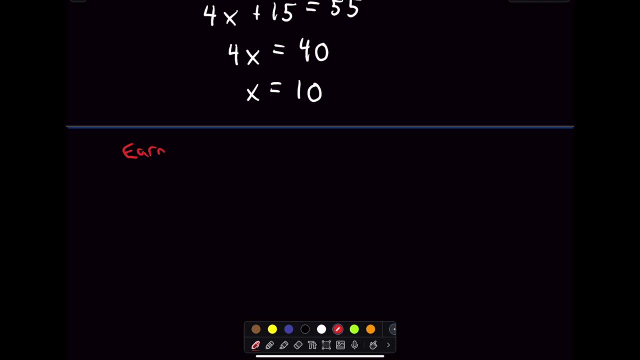 And that simply means: right the earnings, Let's say: And then one, two, three. right, we've now really done the hard part. We'll just take, take twelve dollars, because that's how much each person works, And then we'll just multiply that by the number of hours they worked, which we said was 10, 15 and 30, respectively 10, 15 and 30.. 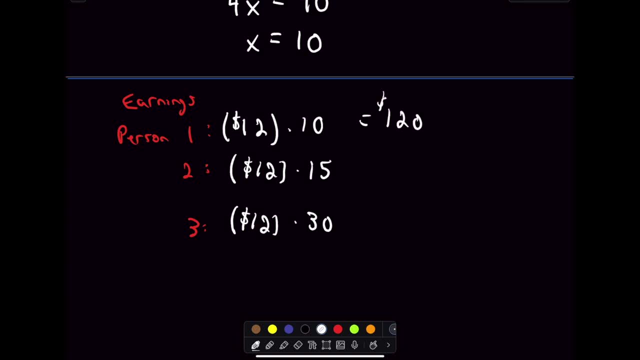 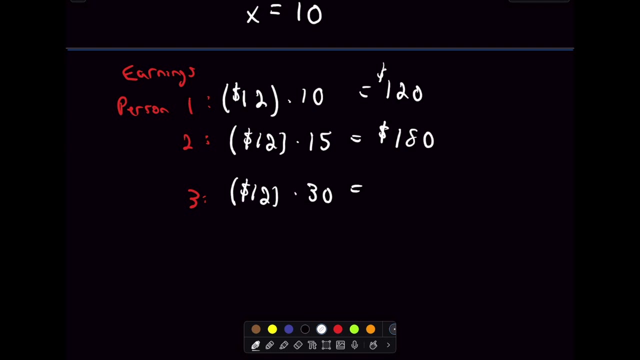 So employee one made one hundred and twenty dollars. Employee two made- What is that? One hundred, Let's see. We said five more One hundred and eighty dollars. There we go. And then the last person made three hundred and sixty dollars.